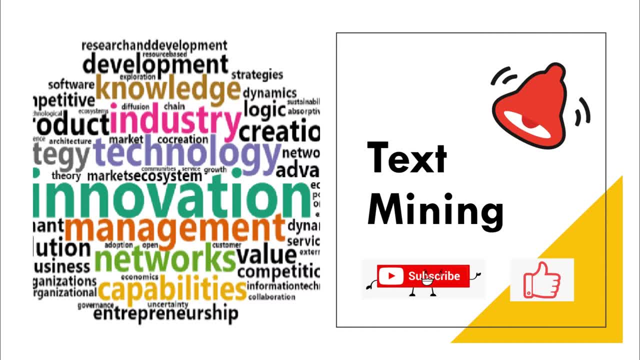 like subscribe and you hit that notification bell if you want to hear more from me, if you want more content on analytics and if you want to learn more about the field. so today we're going to be discussing text mining and we are going to go through theoretically what text mining is about. 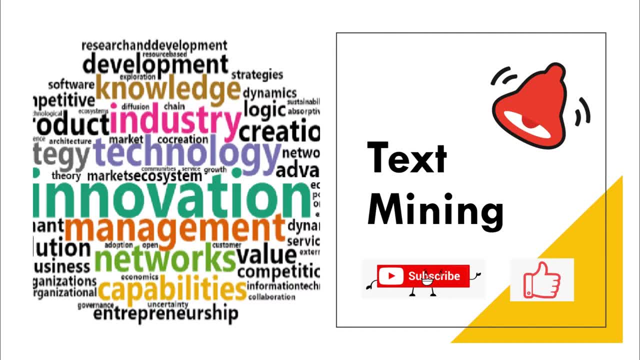 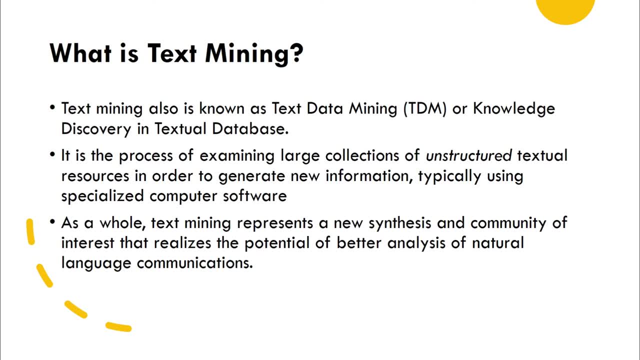 and then we're going to go through an example using R For data mining. we are looking at what is data mining, What is text mining really about, right? So text mining is also known as text data mining or knowledge discovery in textual databases. It's really how you take unstructured textual resources or data to generate information that is typically created using some specialized software. 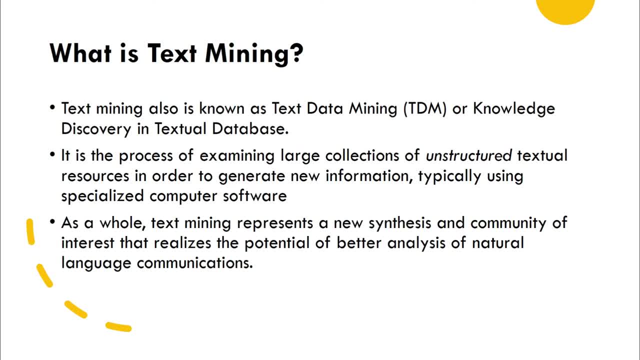 So we're going to touch on the software today as well. On my channel, I tend to use open source platforms such as RR Studio, So that is what I will be using to demonstrate the text mining approach. Now as a whole, text mining represents a new community of interest that it's about realizing the potential that exists in language and communication. 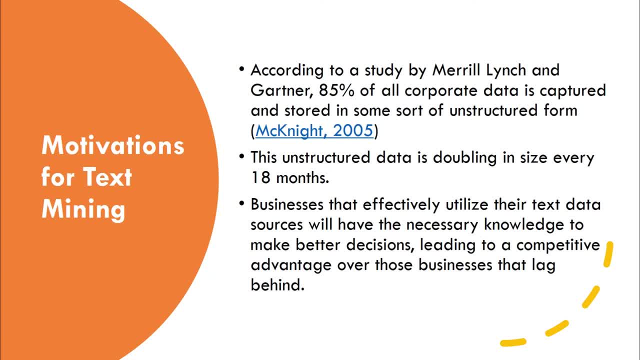 Now, what is the motivation behind text mining? According to Mary Lynn from Gartner, 85% of all corporate data is captured and stored in some form of structured, some structured form or the other. So what are we talking about? We're talking about the company email. we're talking about policies that are written. we're talking about calls coming through a company's contact center. 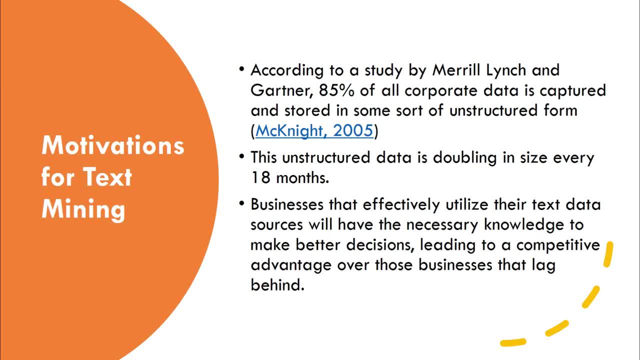 So what is text mining- Or you may be chat being done online. some of the application processes. if you are writing out, you know, descriptions pertaining to an accident with your insurance company. a lot of the content is in unstructured format. 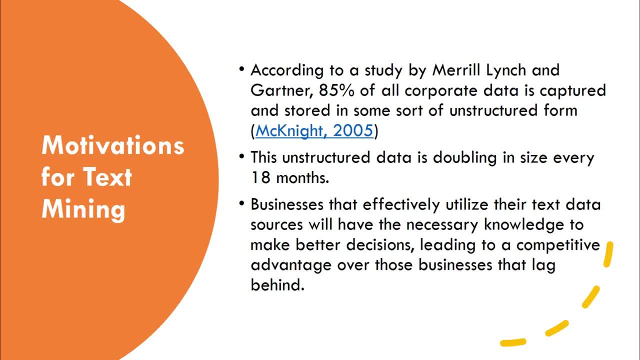 And the truth of the matter is it's not easy to move from unstructured to structured format without having that know-how. now what we see happening is that unstructured data is doubling in size every 18 months, and for me I think it may be happening a little bit faster than 18 months, but 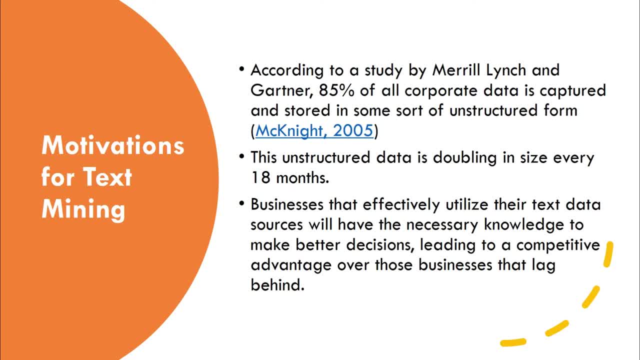 we're going to keep that as a standard. now: businesses that effectively utilize their text data. they will have the necessary knowledge to make better decisions that lead to come a competitive advantage over- you know, other businesses, so they can leave them behind. so what is the goal of text? 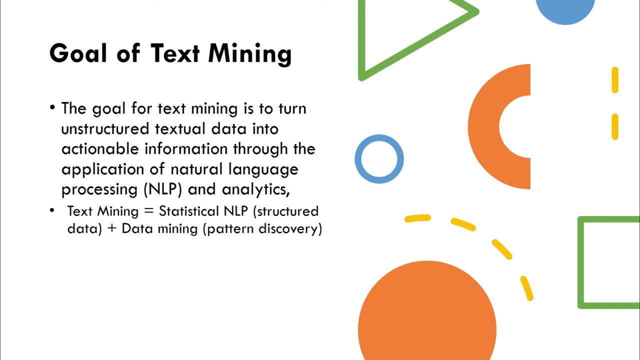 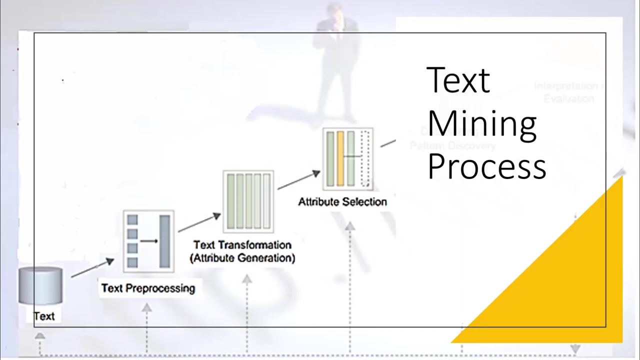 mining it's really to turn unstructured textual data into actionable information through the application of natural language processing and analytics. so text mining really takes advantage of statistical NLP, which focuses on how it can structure the data, and then you have the data mining side, which looks at pattern discovery within the data. so the text 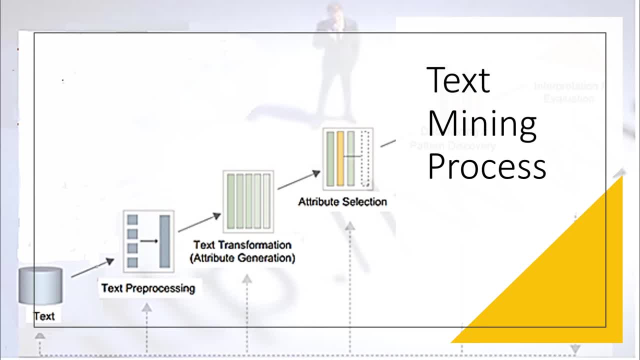 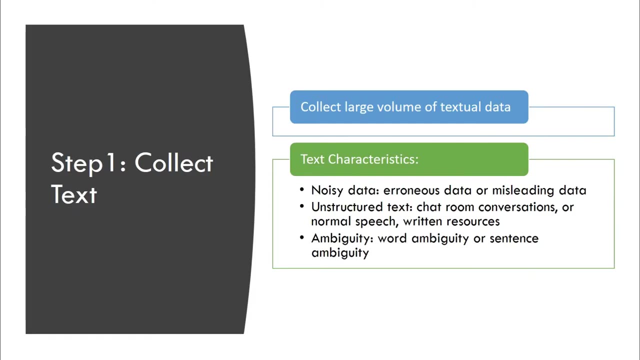 mining process, the steps: are you really collecting the text? you're doing some pre-processing, you have to transform the text in some way and then you have some amount of attribute selection to do your analysis. so I'm going to go through each of these steps. so, step one: to collect text. now you have to collect a. 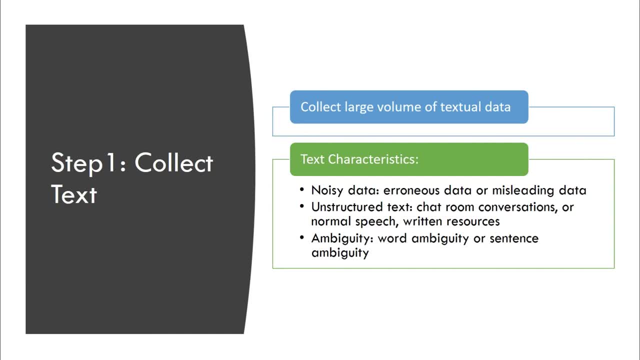 large volume of textual data, really because you're looking for certain patterns and you need enough data to identify those patterns. but there are some peculiar characteristics pertaining to text. data is noisy, right, and textural data is part of a classical class and text is not a often used and it's not a. 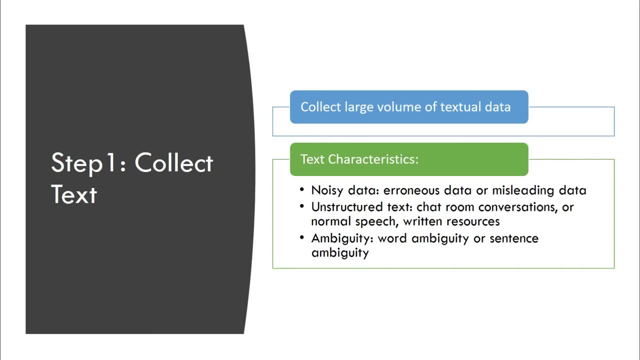 particularly noisy. When I say noisy, I mean it has a lot of errors. It could be misleading data as well. Data is also unstructured, So if you're analyzing data coming from chatroom conversations or regular speech or written resources, there's not going to be a very 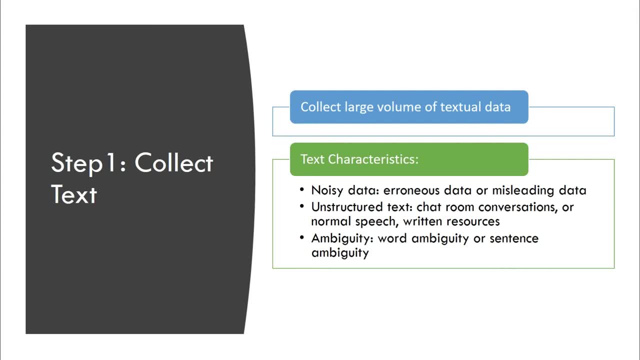 visible format in terms of how the data is represented, in terms of that structure. There's also the issue of ambiguity in terms of what words mean. So, for example, when we look at text, when I see the word apple in a text, is it apple, the company, or is it? 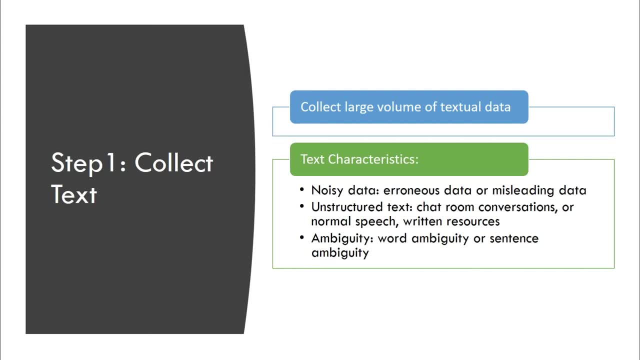 apple, the fruit. So that creates some amount of ambiguity, not just the word, but the word. So when I say the word, I mean it has a lot of errors. So if you're analyzing data coming from chatroom conversations or regular speech or written resources, 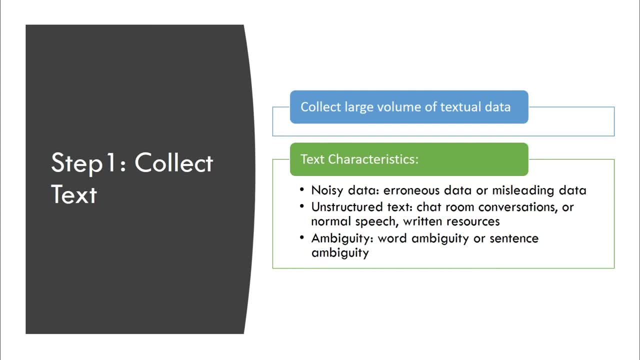 that culture has some impact on data itself. So, for example, I am from Jamaica. We have certain terminologies or a certain way that we speak that we may impact the original meaning for a word. So, for example, when we say that body, we don't necessarily mean that something is. 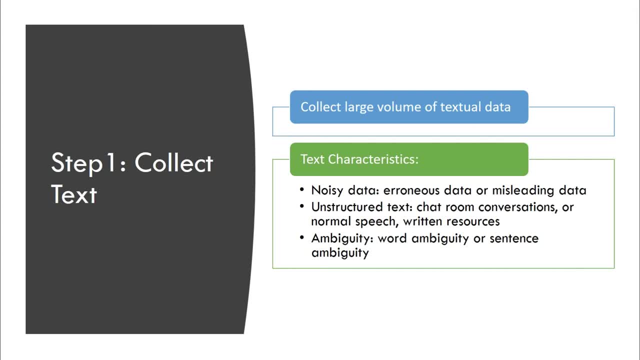 bad in a negative way, We may actually mean that it's good. So when persons use certain terminologies like that that is impacted by their culture, or that's lit or that's on fire, fire may be considered something negative. However, the word fire used in that context may be a positive. 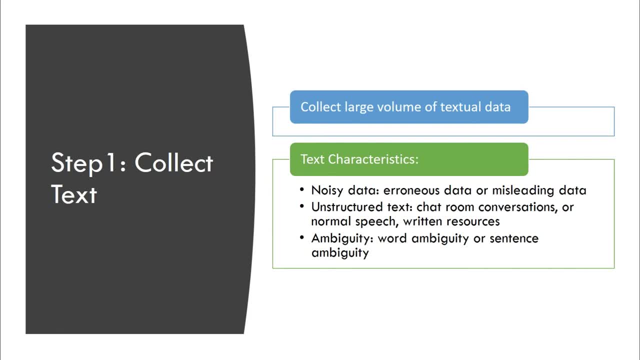 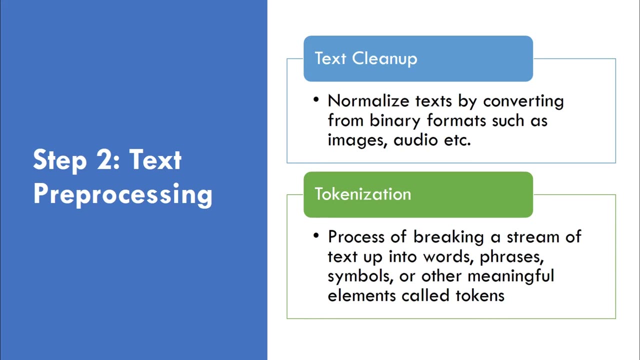 word in that particular sentence. So there's some amount of ambiguity sometimes that is used in text And of course, that ultimately impacts your analytics. So once you've collected your text, step two is really the processing of the text. Now you must do some amount of cleaning up, which means you're converting from binary formats. 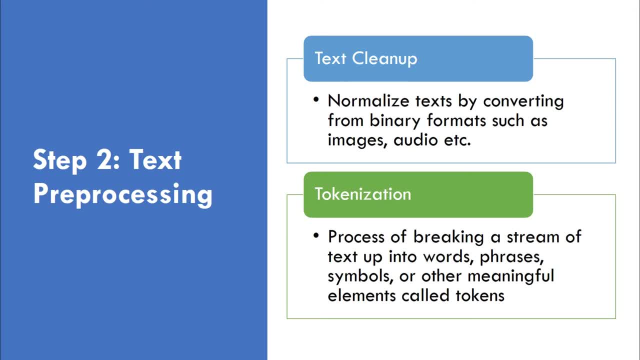 such as image, audio et cetera, to what we call tokenization. You're creating tokens, So tokenization really is a process of breaking a stream of information into a text, And that's what we call tokenization. So you can create a stream of text into words, phrases, symbols, et cetera. 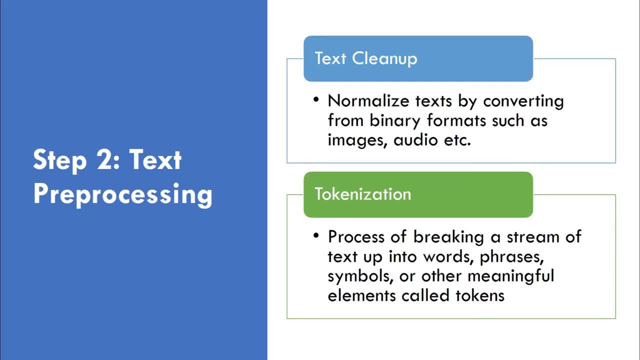 And what you want to do is to ultimately find meaning or do some processing for these tokens. So, for example, if I had the text this is a ball, To create tokens would mean to break the sentence up. This is a ball, with this being a token. And then you can create a token with this being a ball. 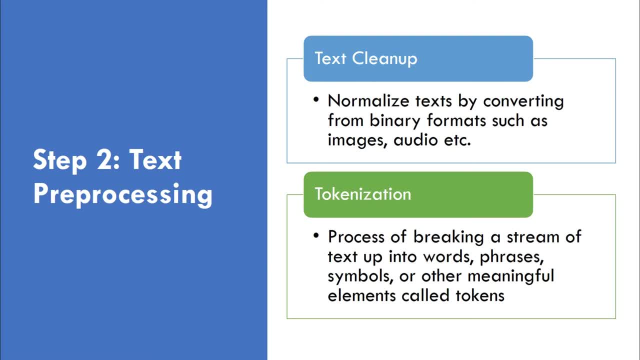 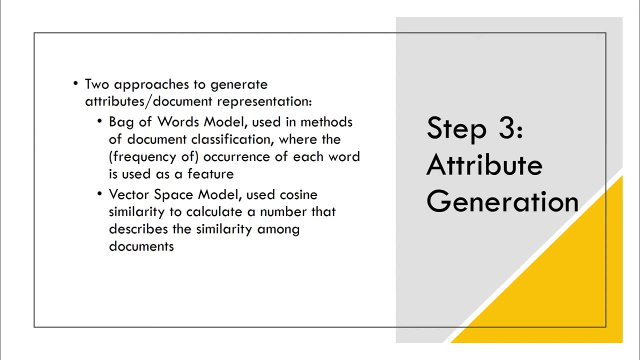 So when we talk about tokenization, we're talking about breaking up a sentence into different pieces. The next step is what we call attribute generation. So attribute generation is there are really two approaches, right, And you are trying to identify the different attributes. 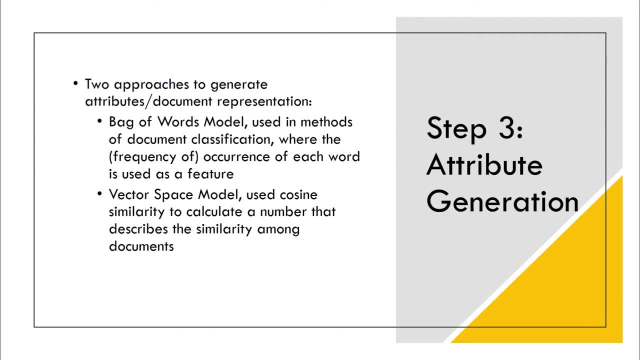 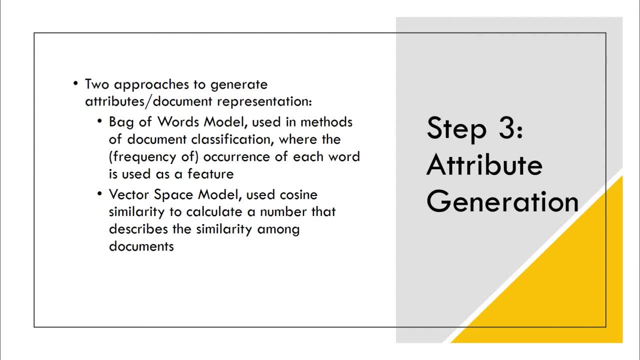 for example, the frequency of the words. How often do you see a word appearing in a particular text? And you can use that to get a sense of you know what this text is really talking about. What is it in reference to? How often do you see this word appearing? So bag of word is one approach. 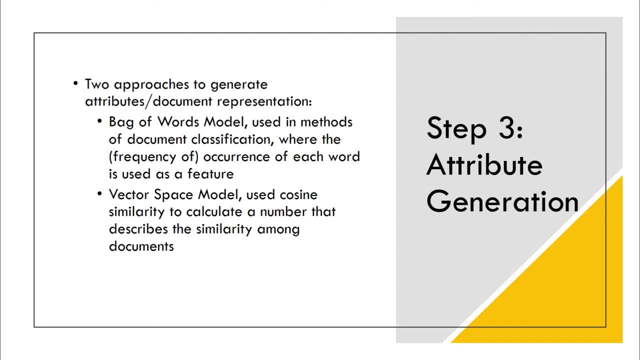 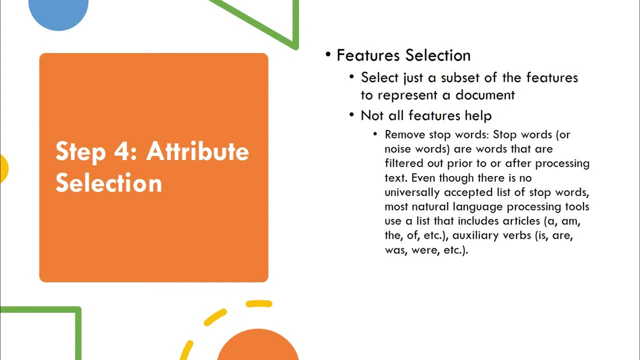 There's also the vector space model, where you use a cosine similarity to calculate a number that describes the similarity among different documents. Now step four is attribute selection. Now here you're selecting a subset of the features to represent the document, So not all features help right. 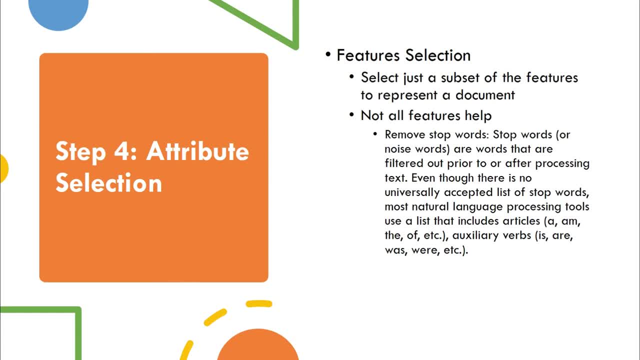 So not all words in a document help to understand what the document is about. We have what you call stop words. Now, stop words or noise words. they're words that you want to filter out prior to the processing because they don't really contribute to. 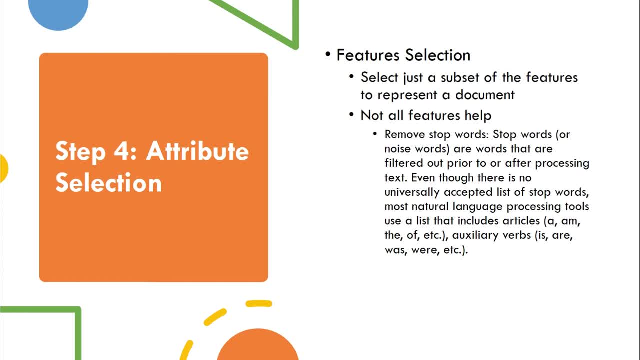 understanding. So, for example, the was, is, are, am, you know they, those are stop words and we have some universally acceptable list of stop words that are used to remove from an article. Of course, again, culture what I've seen in the past in analyzing certain documents. 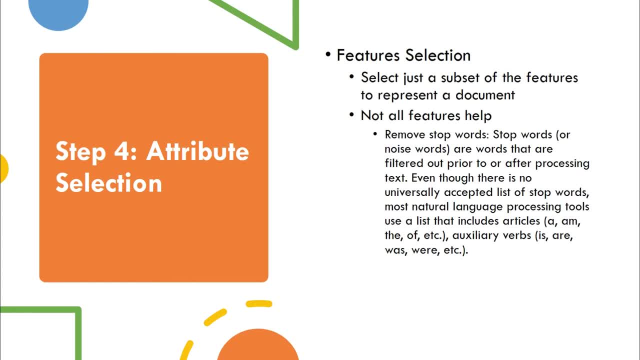 is that culture may impact the type of stop words that may be acceptable or not. So you have the basic stop words, but after going through your document there may be some words that are not really useful that you would love to to take out, And there's some. 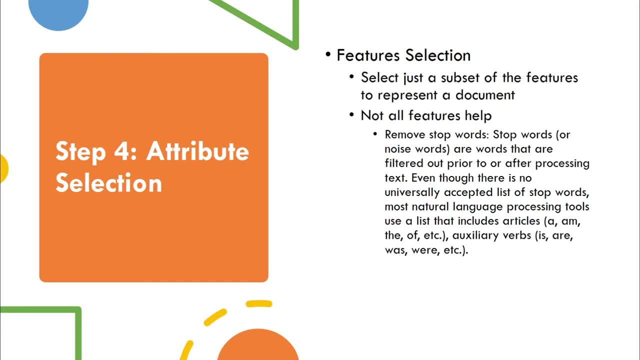 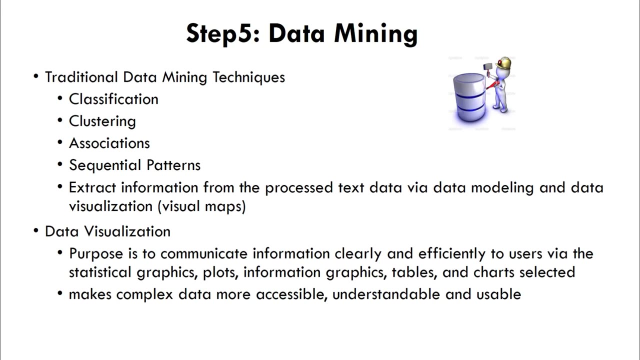 technology that would allow you to improve on words that you can have removed from the documents. So that's what attributes selection is all about. Now, once you've gone through that whole cleaning process, you know you've removed your stop words, et cetera. The next thing: 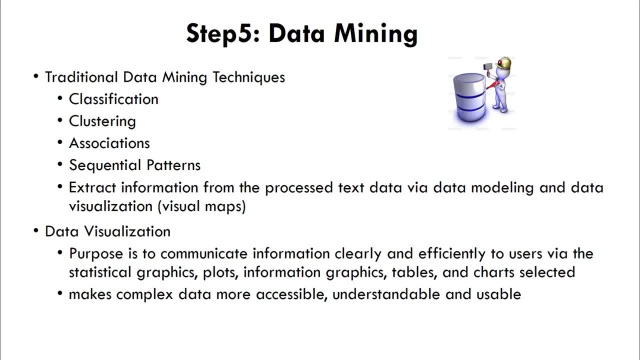 you're going to want to do is you're going to want to remove your stop words. So you're going to want to sort of remove them. you can, if you want them to, to be little bit smaller than an active concerning words. You know, if they have that's that specific thing that will. 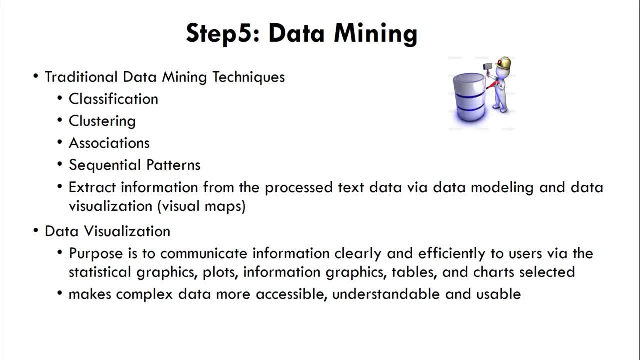 have, multipleasmine are ones, so you can sort them in 0.1 of terrain. So you're going to want, you want to remove all the stops in order to be not история. you want them to be, you know. 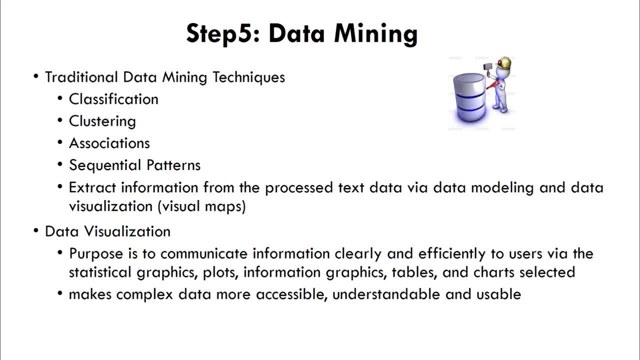 вам to keep it constant that don't have a complete until when I take a typo out of my tables, charts, etc. so we're going to touch on some of these things, um, in this particular lesson. so we will be going into our and just walking through to determine, you know, how will we? 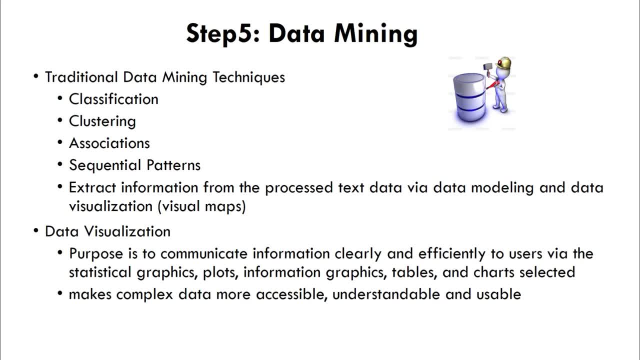 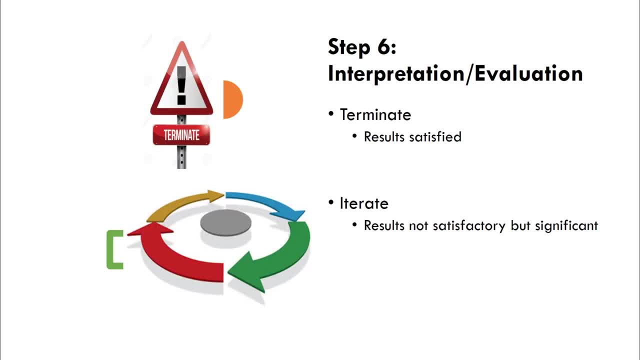 explore text mining um in our to see exactly how it works. now the final step: interpretation is important. now you're not only just creating text, but creating text analytics for the purpose of just doing so. your results must be interpreted. it must be applying to a situation. now, when you get to this step, you're either going to terminate because you 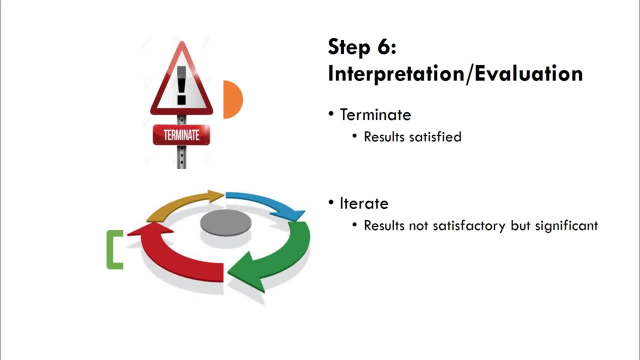 have gotten all the results that you need and you're satisfied, or if you're not satisfied, there's going to be a process of iteration and you go back through collecting more data until you reach that step where you are indeed satisfied with the results. i find sometimes this is where a lot of data scientists or analysts 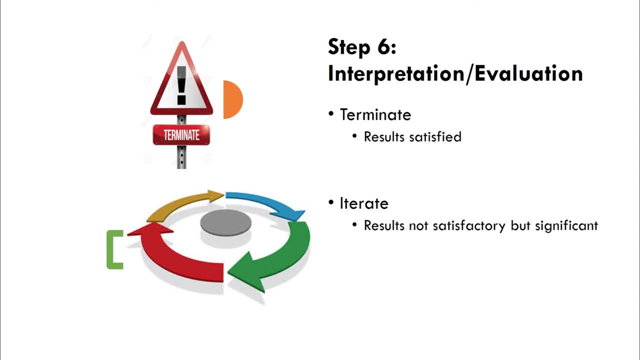 struggle in interpretation phase or evaluation phase of any data mining exercise. i'll do another video that speaks about the importance of understanding a business domain, because purely understanding how to execute a particular data mining technique is not enough. you also need to understand the business domain. so the first thing is the package that we 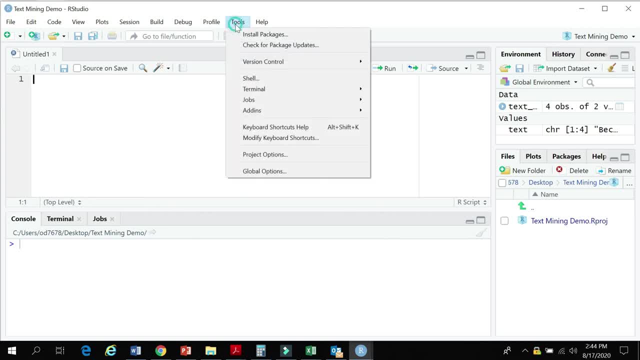 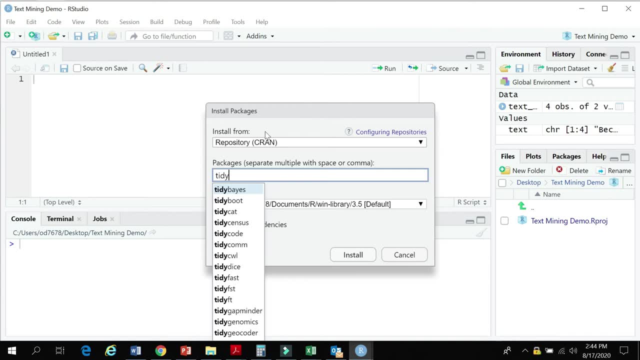 need? we need a package called tidy text. so you have to go to tools- install packages and you search here for tidy text. now, i'm not going to install it, it takes some time. i already have tidy text, so i don't have to go ahead and install, but this is where you would find it. you also need another package called. 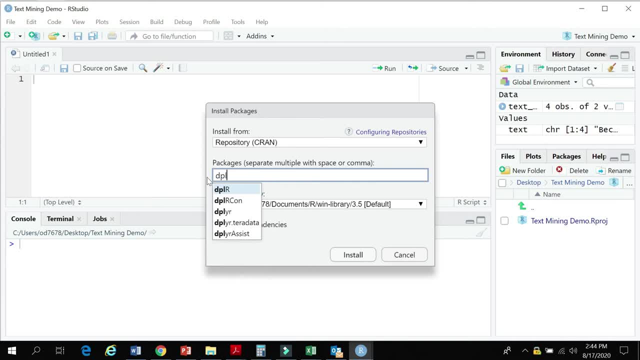 dp l y r. this is it. you need to install that as well. i already have it installed, so i won't go ahead and install it again. so you need those two packages now. you have to tell r that you want to use each package, so use the, the keyword require, and you want to require the tidy text package. 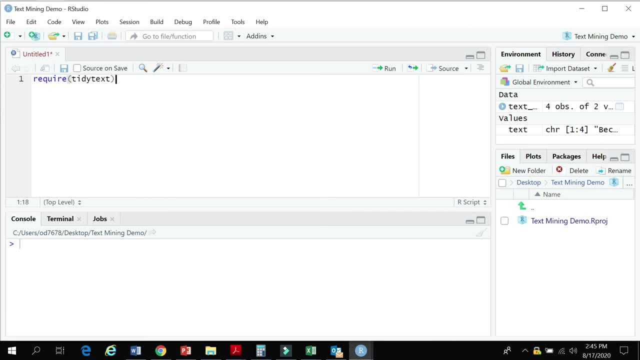 and this is so I like to put comments to just more remind myself of what each line of instruction or code is doing, and also for those persons who are learning for them to you know, know that this is exactly what the instruction does. so this is the package: you to tokenize words. and then we also need to require 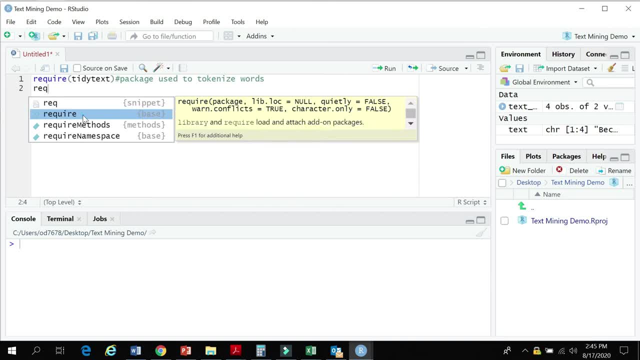 and you see our studio suggesting it, so hit require require that. you see our studio suggesting it, so hit require require that dplyr package, and this is the package that we need for data frame manipulation. all right, so package for data frame creation. all right, so you can go ahead and just highlight these two lines once you install the. 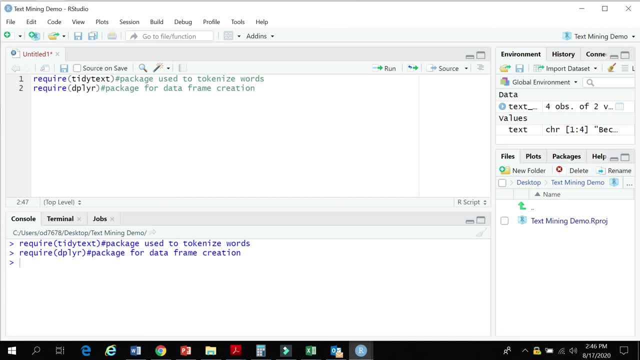 packages. you highlight these two lines and run and, if all is good, you're going to see um, the line in blue down in the console. so now the next thing is that we need to create um, the vector that is going to be used to store the results. so i'm going to store it in a variable. 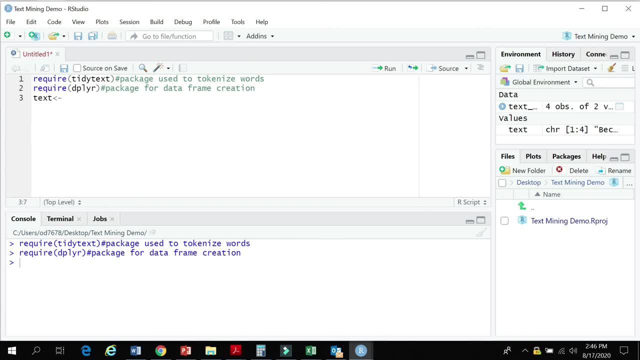 call text and in text. so this symbol here is the less than, followed by a minus sign. um, we are going to type what we are creating. so this is the poem. because I could not stop for death in quotes, he kindly stopped for me. comma. next line: open quotes: again the carriage held, but just for ourselves. 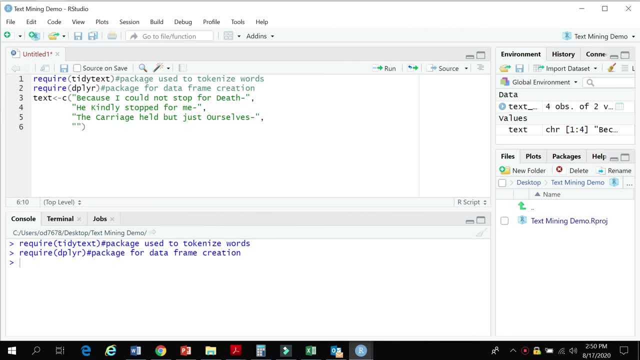 alright, so the next line and immortality. so that's our poem, that we created a vector so we can run, and all it's. well, we see the lines coming up below here in the console in blue. so I'm going to put a comment here that says creating: 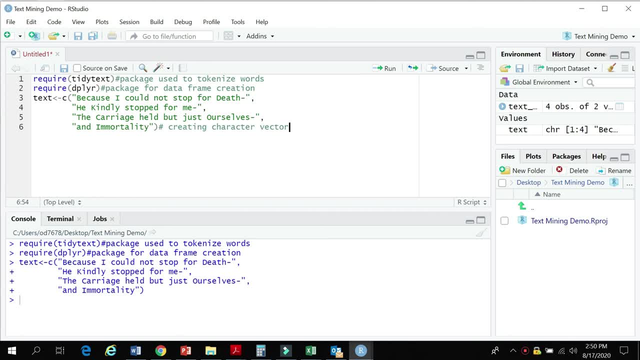 practical vector. right. so then the next thing. so we, if we highlighted text, only here we will see what's in text, that this is a variable where we stored all the lines for the poem. so that's it. so the next thing is that we must know convert the vector into a data frame. 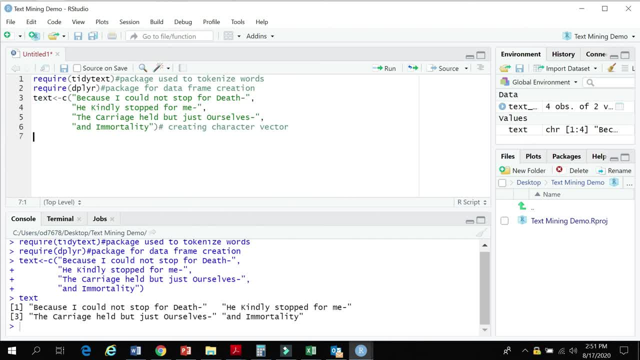 so that we can create tokens out of the flop. so let's go with our view. considerable check on the Stoke, even if bent for me, cuz that was the sound of four 복 духs were. so we're using the command data underscore. friend, I'll leave it to you to upload your topic. let's write it in the comments, byготовichgarou and a. that's it. so please don't forget to share this video. 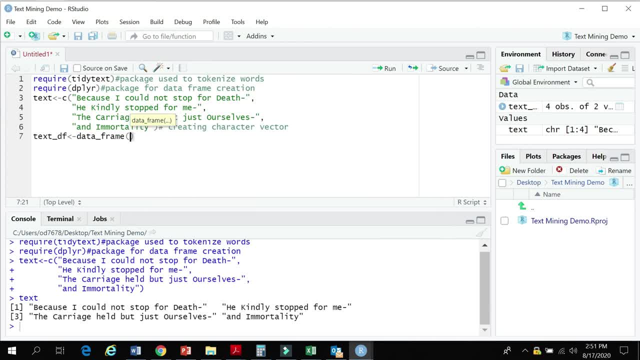 Alright, we want the first one and it takes the argument's line. So here we're specifying how many lines a quorum has and we're using equal one, two, four comma and we're converting text to text. All right, so comment here: converting vector into data frame. All right, you can go ahead and run that, All is well. 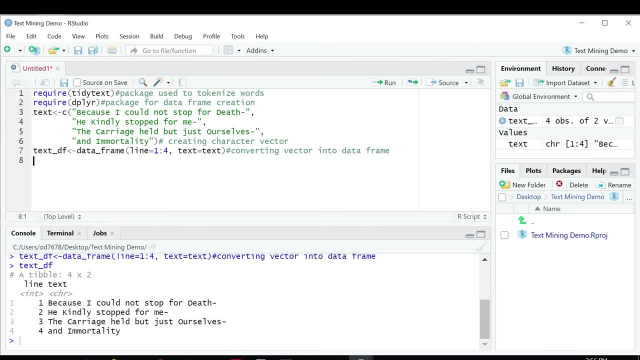 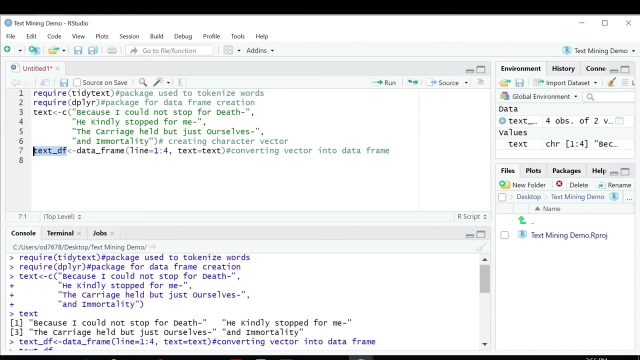 It shows what's in the TX data frame. If we run that, we're going to see here. it's more structured as the data frame. It shows a data frame with the labeling of each line, versus what it looks like when it was just a vector. 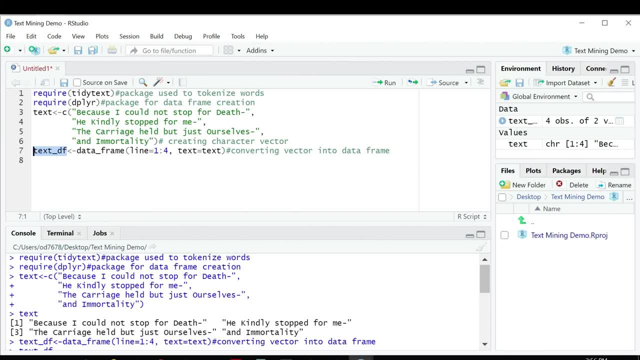 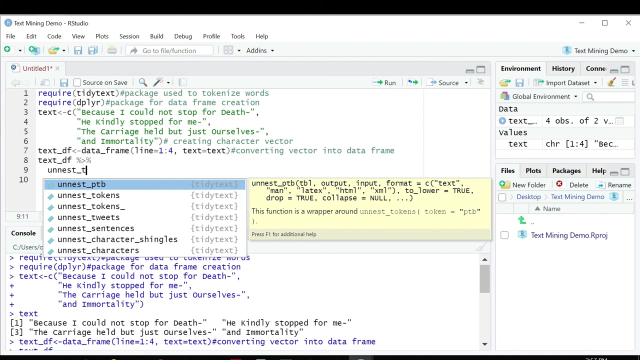 All right. so the final step is that we want to break this up into tokens, So we use text underscore DF, percentage greater than percentage enter and we're creating underscore, Nested underscore tokens, All right. and we want to break it up in words, using text.